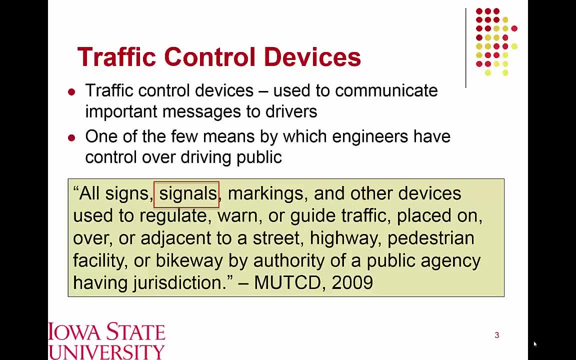 which would include traffic signs, traffic signals, pavement markings and various other types of devices that are used to regulate traffic, Provide warning to motorists and then also serve as guidance, And so the focus of this lecture will be on traffic signals, which are one of several types of different traffic control devices. 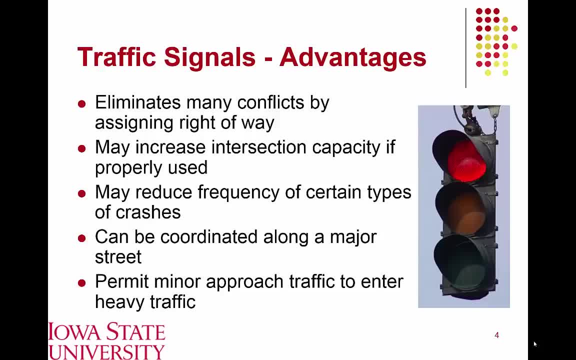 Now, traffic signals have several potential advantages as compared to other intersection types such as two-way or all-way stop control or yield control locations. One of the big advantages is that it eliminates potential conflict points. So say, for example, you have a vehicle that's trying to turn left from a minor road onto a major road. 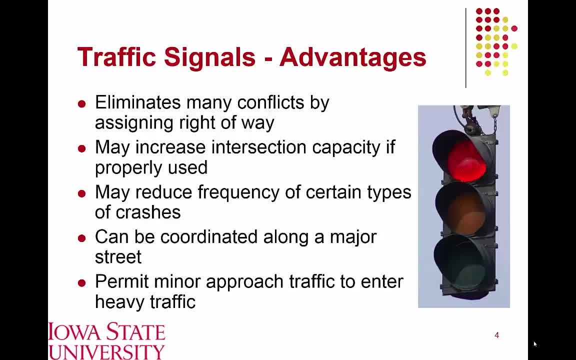 They would generally have to wait. They would have to wait for gaps in traffic, And if traffic volumes are particularly high it may be difficult to obtain those types of gaps. So a traffic signal, of course, would provide a natural stop for some of those vehicles. 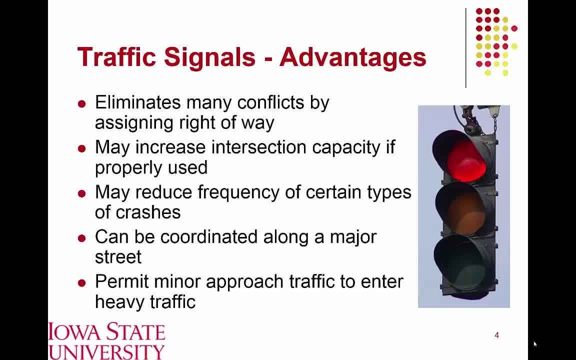 and allow traffic from the lower volume minor street to then enter the intersection. Under certain circumstances, capacity tends to be increased at intersections. if we go to a traffic signal versus stop control, depending of course on the traffic volumes, We may see reductions in certain types of traffic crashes. 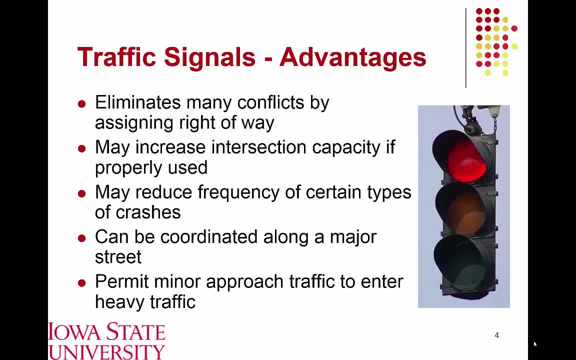 when traffic signals are installed. A big advantage is that we can install signals along a specific corridor and we can coordinate those signals so that as you get from one signal to the next along a major street, we see you're able to hit each of those successive signals, on the green phase, for example. 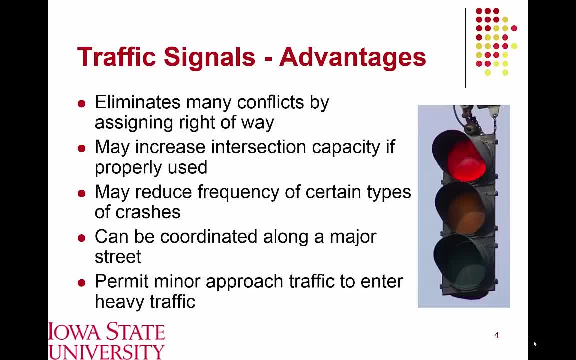 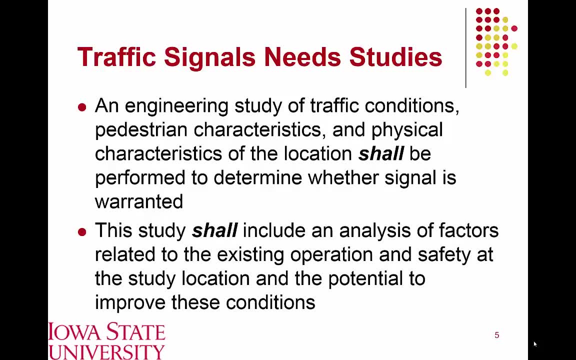 And then, of course, traffic signals also allow minor traffic to enter the major roadway, as alluded to previously, where otherwise that may potentially be difficult. A natural question we run into is traffic engineers is: well, when is a traffic signal actually warranted at a given location? 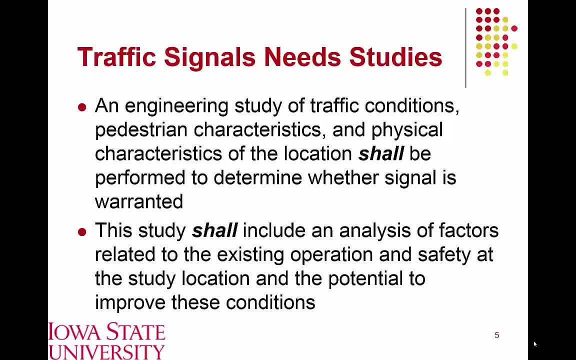 And so the Manual on Uniform Traffic Control Devices, or the MUTCD, essentially recommends that a traffic signal needs study should be conducted prior to determining whether a signal should be installed at a given location, And so these traffic signal needs studies should consider both traffic operations as well as safety. 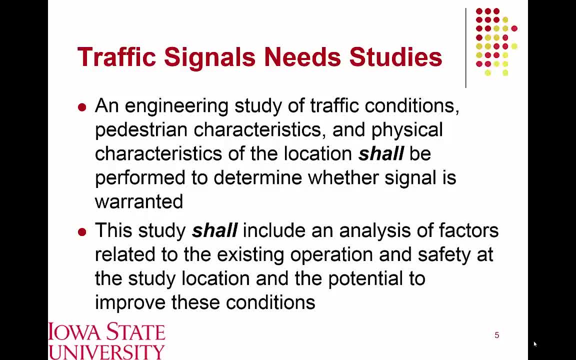 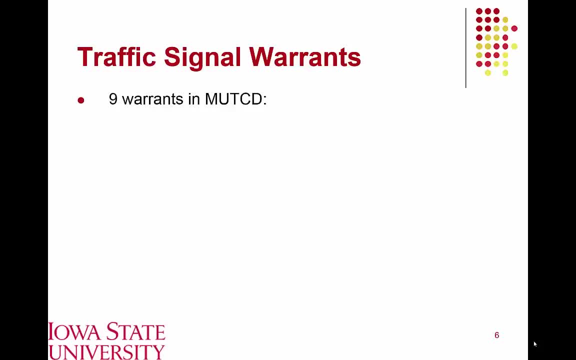 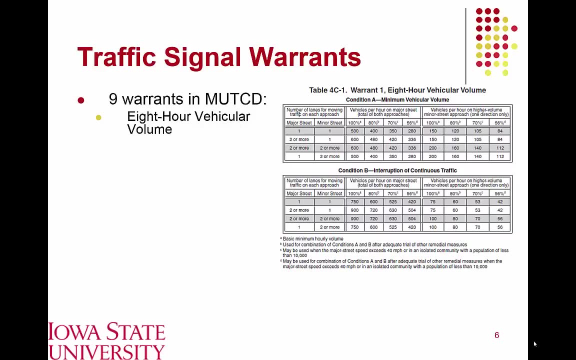 and what the expected impacts would be as we transition from, say, a two-way or all-way stop to a traffic signal. The MUTCD outlines nine specific warrants under which traffic signals present a potential solution. These are generally based on traffic volume, vehicular volume particularly. 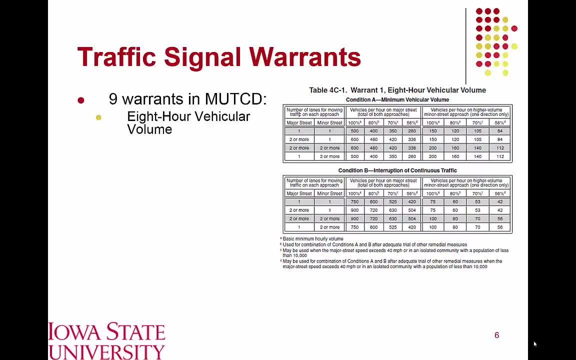 and so the first of these warrants is an eight-hour vehicular volume warrant. So, essentially, you look at the highest eight-hour period at a given intersection over the course of a day. We look at how much traffic is using the major street, how much is using the minor street. 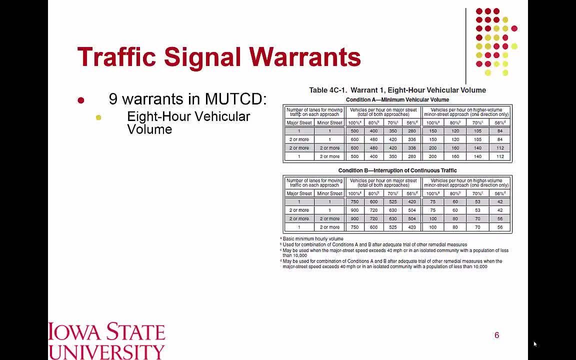 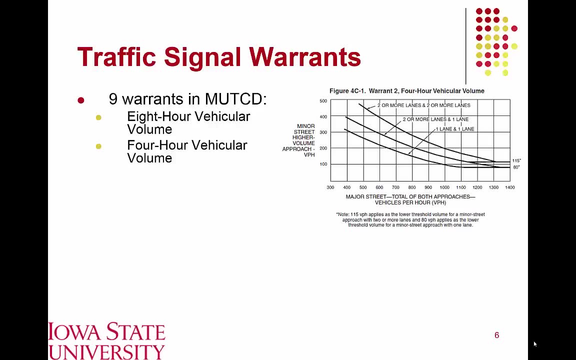 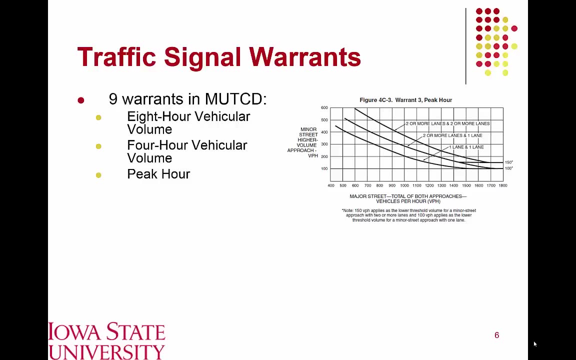 and on that basis we make a determination as to whether or not a signal may be warranted. Likewise, we can look at shorter time periods, so looking at the highest four-hour volume in consecutive hours along both the major and minor cross streets, or we can narrow that down simply to the peak hour period. 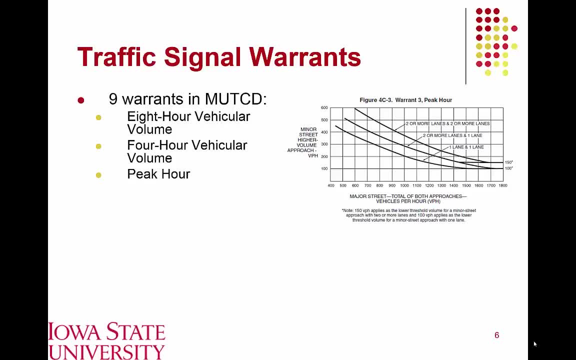 So we look at the highest one-hour volume period during the day, see how much traffic is utilizing the major and minor street, and then make a determination on that basis as to whether a traffic signal is a viable alternative. While each of these focuses on motor vehicle volumes, 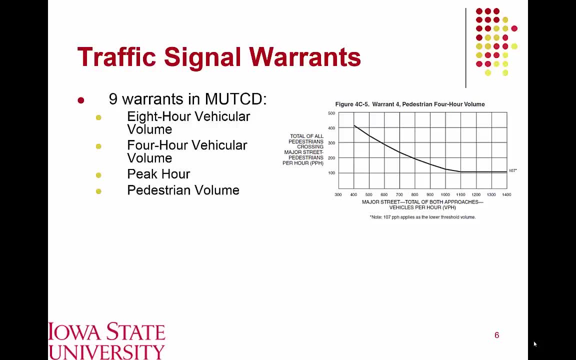 we also want to be cognizant of pedestrian volumes. So if you have heavy ped activity and that ped activity is introducing a lot of delay for pedestrians, given most of the time signal timing being prioritized towards the motor vehicle traffic, we can look at installing signals on a basis of these pedestrian volumes. 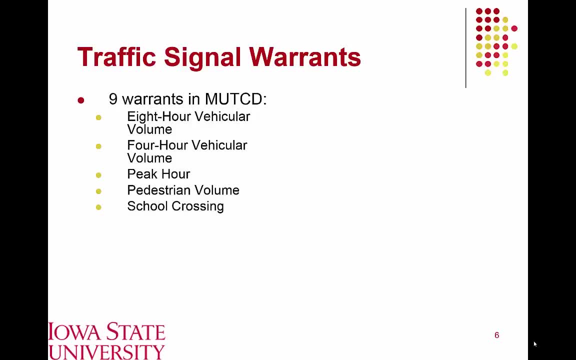 A special case of that warrant would be in the case of school zones. So if you have school crossings, you have a large number of school-aged or young pedestrians. that would be a circumstance where we'd want to look at trying to potentially consider a traffic signal. 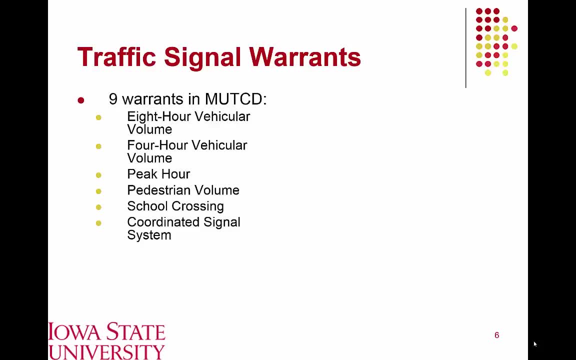 Coordination. so if you have a series of other traffic signals along the same corridor, introducing another signal and trying to coordinate that so that you're able to go through each of these successive signals under green is, of course, going to be a potential advantage. 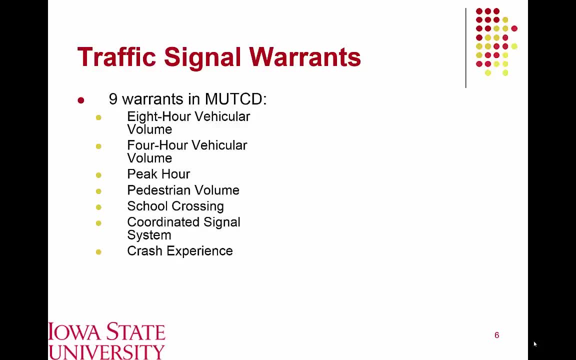 Crash experiences. so there's certain types of crashes, such as when vehicles are trying to turn left from a minor street onto a major street. that can be problematic if there's not a traffic signal in place. So if we have a history of these types of high-risk collisions, 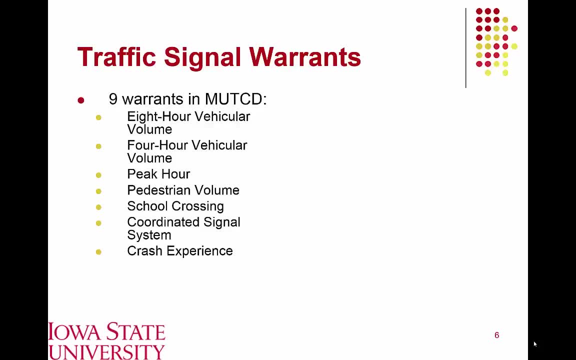 that would be one potential indication or a warrant for traffic signal consideration, And then also looking at the characteristics of our road network and what other intersections may have traffic signals on that road network, And then lastly, whether or not that intersection is located near a rail grade crossing. 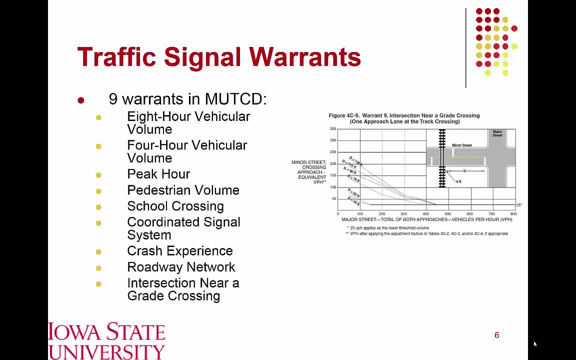 So let's say we have major and minor, minor streets with specific volumes and there's a rail grade crossing nearby. A signal may be warranted here to ensure that traffic does not get backed up onto the railroad tracks, for example. So this is an example figure coming out of the MUTCD. 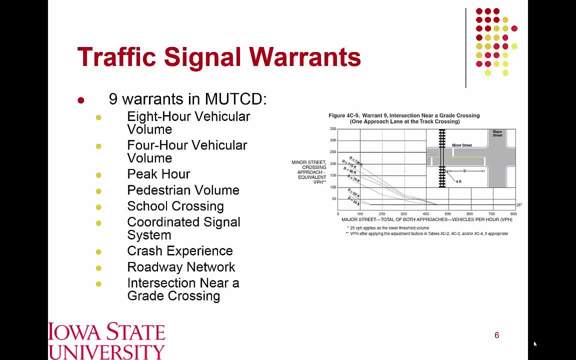 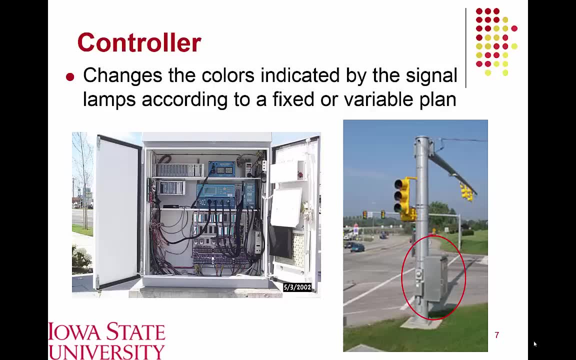 that indicates when a signal may be warranted under that condition. So when we look at the actual traffic signal and its operation, the signal is going to be operated through a controller which is going to be located in a cabinet near the roadside, And so here you see an example of a controller. 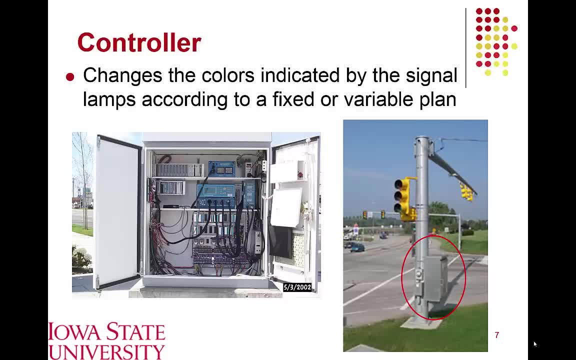 which is located in this cabinet, which has been opened up for view here, And so what we're going to do as traffic engineers is we'll try to develop signal timing plans that will be implemented through this traffic controller, which is located in the signal control box. 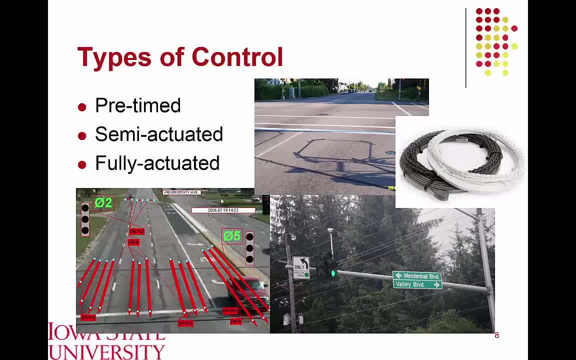 Now, when we're operating traffic signals, there are three general types of control or traffic signal operations, And those include pre-timed, semi-actuated and fully actuated. And so these traffic signals, for those types that are actuated, 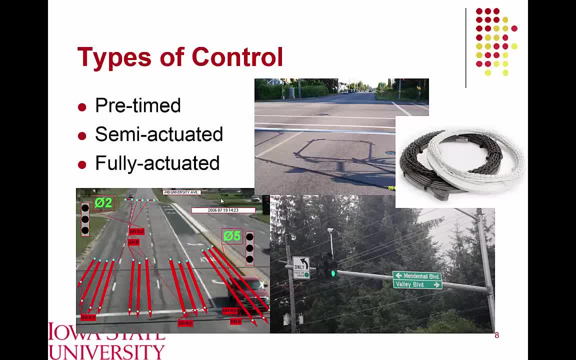 those devices are basically activated by some form of detection device, whether that be a loop detector that's located underneath the pavement, or we've seen more progress recently going towards video camera-based detection, which would involve overlays of the video detection, as you see indicated in the bottom left here. 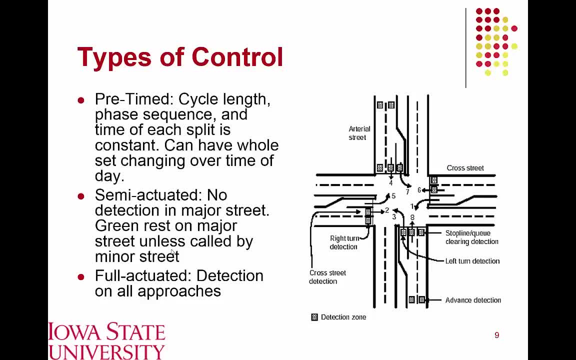 Now when we look at these three different types of control. pre-timed essentially refers to intersections that are operating on a fixed cycle length, So you have the same fixed amount of green, yellow and red for both the major and the minor street over a given time period. 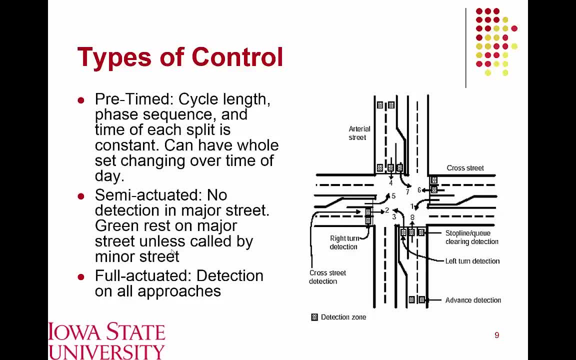 And you could have an intersection that operates under the same pre-timed cycle length throughout an entire day, or you could see some variability throughout the day. For example, you may see a different timing plan during the am or pm peak period versus the off-peak periods. 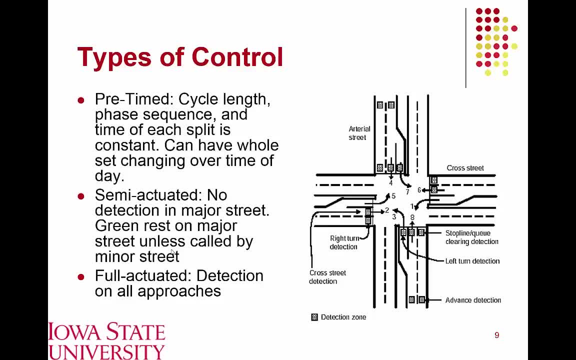 In contrast, actuated control. semi-actuated control refers to the circumstance where you have traffic on the minor street that's trying to enter the intersection and either cross or turn onto the major street And under semi-actuated control we basically give green time. 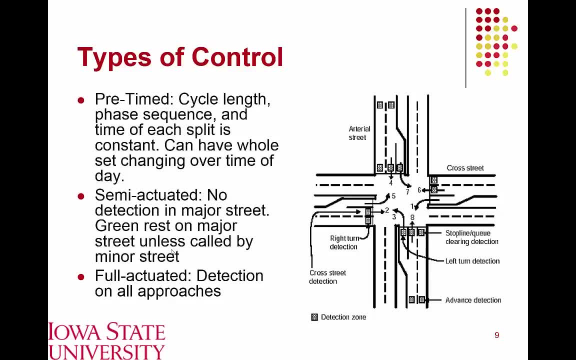 to the major road exclusively, and we only provide a green signal for the minor street if there's actually traffic waiting there, which is detected and then sends a signal to the controller cabinet. Going one step further, we also have what's referred to as fully-actuated control, where we have detectors. 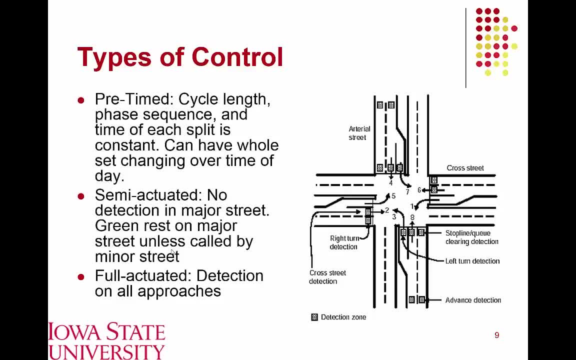 on each of the approaches on the major and the minor road, And so this is not just sending signals that hey, we have a vehicle waiting here, but also these detectors can help us to inform the controller as to when to terminate specific signals as well. 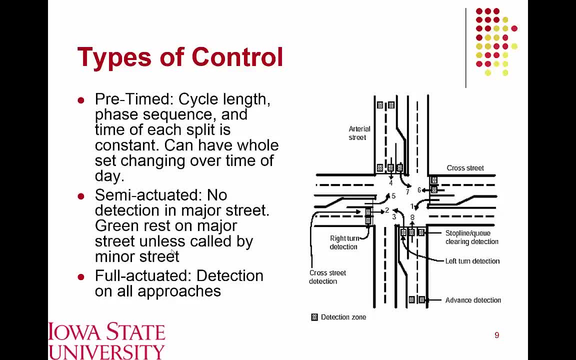 So we'll start talking about some of these nuances in greater detail as we get further into the course. But for the purposes of CE 355, we'll primarily be concerning ourselves with pre-timed traffic operations. So in this setting we can conceptualize this time-space diagram right here. 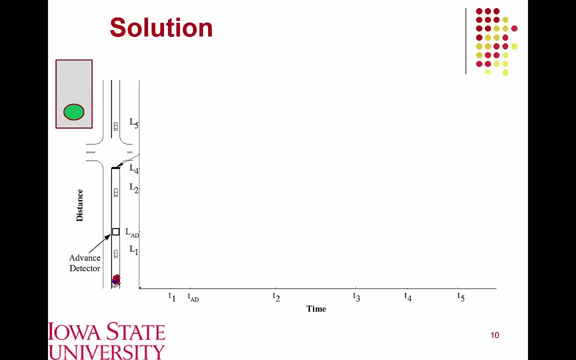 where, let's say, on the y-axis we have a distance at a vehicle is traveling as it's approaching a traffic signal, and on the x-axis we have time that corresponds to this vehicle's trajectory, And so what we can do is we can plot out that vehicle. 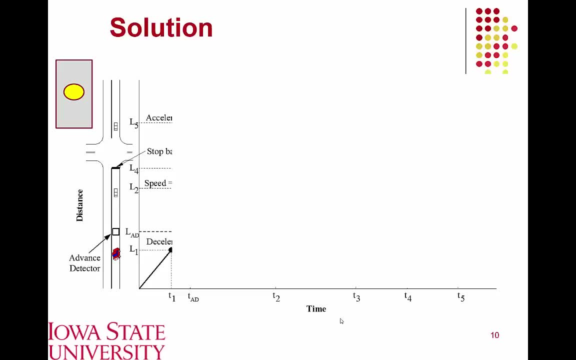 as it's approaching a green signal that's about to turn yellow. The slope of this line is giving us an indication of the speed of that vehicle and we'll see once the driver recognizes that the signal has turned yellow, it'll begin decelerating. 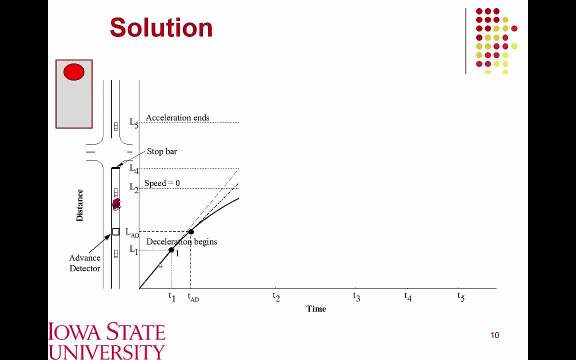 and it will continue decelerating until it reaches a complete stop in advance of the stop bar, And then that vehicle will stay stopped as indicated by this flat trajectory you see, from point two to point three. The signal then turns back to green and you'll see that vehicle. 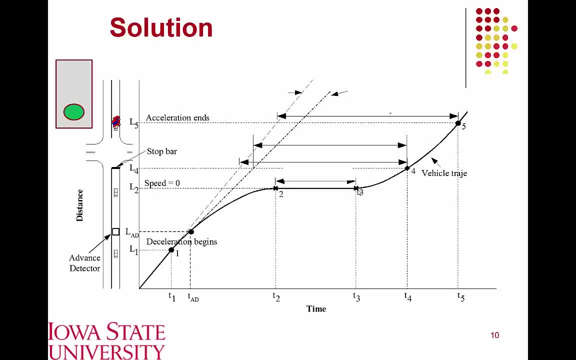 start to slowly accelerate. It begins accelerating until it gets back to its initial vehicle speed trajectory out here past point five. And so if we look at a few of the key points here, so that initial vehicle speed trajectory, as that vehicle was traveling at its constant speed, if we were to project that out, 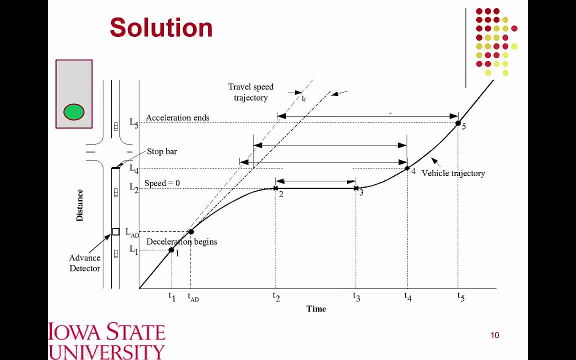 assuming that that vehicle has seen a green light during that entire signal, that's the initial travel speed trajectory. The measured speed trajectory, or what that vehicle is actually doing if it continued through the intersection, would correspond to this point of deceleration, right here. 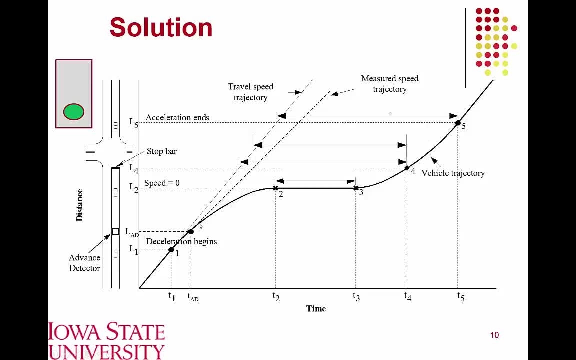 So that vehicle decelerates and then needs to make the decision of whether or not to stop If it decides to continue through. we would then instead observe this speed trajectory. From this diagram we can also estimate several of the important delays, or we can determine how these delays can be quantified. 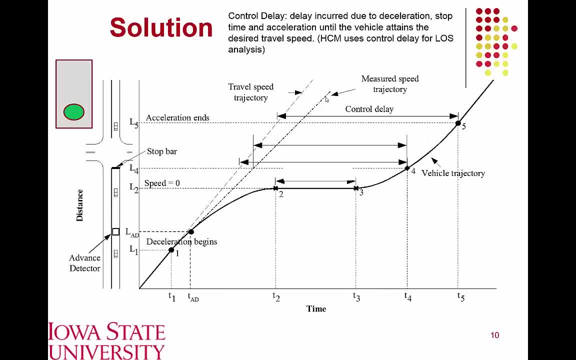 For the purposes of capacity analyses, as we would see in the Highway Capacity Manual. we're going to be concerned with control delay, which is indicated right here by this metric, And so control delay is essentially counting for the time that delay is introduced to the motorist due to them having to decelerate. 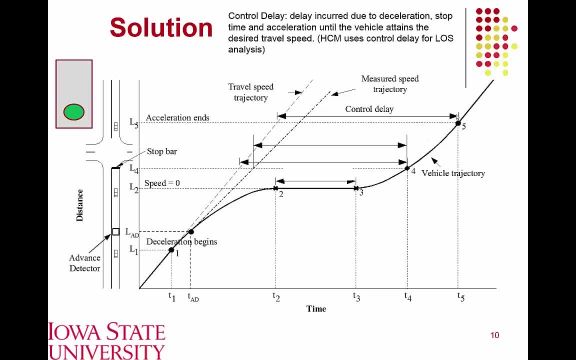 to have to stop and the entire duration during which they're stopped, and then also the time required for that vehicle to accelerate back up to the initial desired travel speed, That's, the speed that they were moving at. In addition to that, there are a few other types of delays. 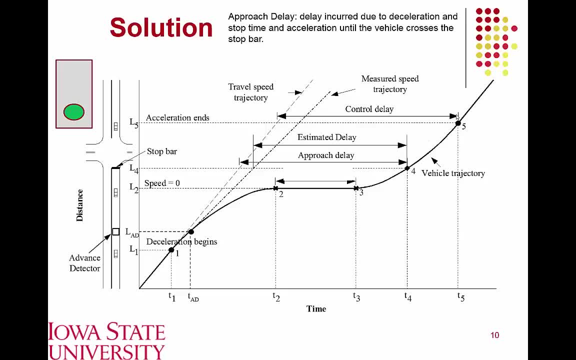 that we are often concerned with, one of which is called approach delay, And so approach delay includes that deceleration time, the stop time and then the time it actually takes for that vehicle to clear the intersection. So this doesn't quite go up to the point where that vehicle would be returning. 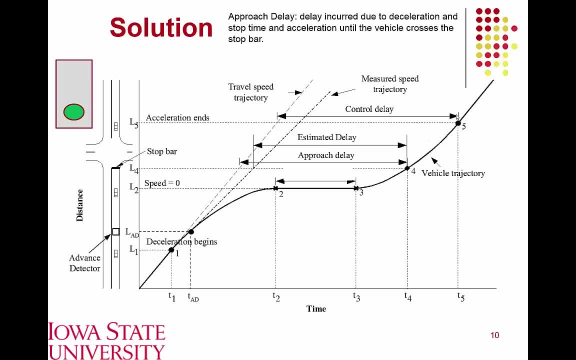 to its full travel speed trajectory. as we see under control delay, It's just capturing that time of delay from when the vehicle encounters the yellow signal on the approach to when it's able to then enter the intersection and cross the stop bar And then, lastly, stop. delay is simply measuring the time. 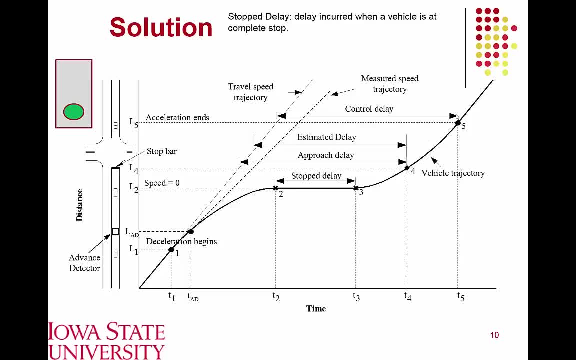 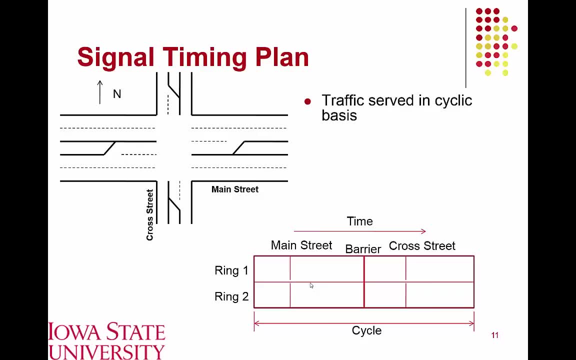 that that vehicle is stopped due to a red signal at the given intersection. And so, ultimately, what we're trying to do with our traffic signal timing plan is to develop a strategy which is going to minimize the control delay that was illustrated on that prior time-space diagram. 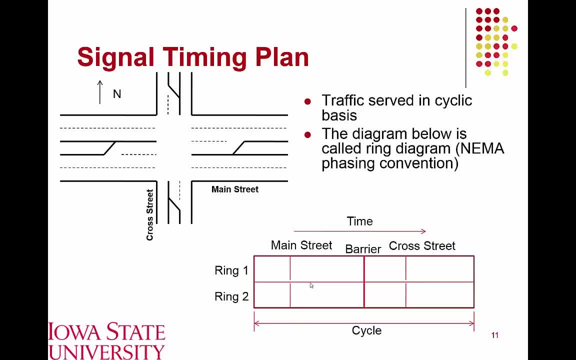 And so, to do this, we're going to introduce what's referred to as a ring diagram down in the bottom Right corner of this slide, And so, in developing this ring diagram, we're essentially trying to determine how much time to distribute to the green, yellow and red movements. 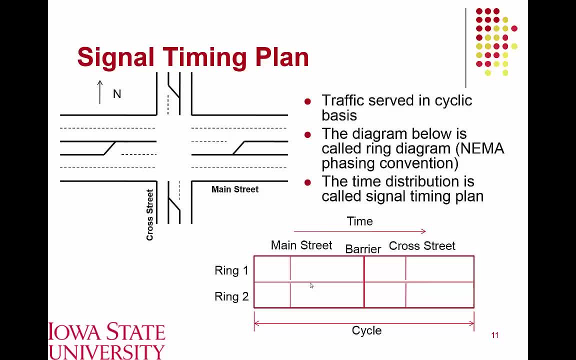 on each of the streets. And so we start by applying a numbering system to these different movements within the signal timing plan. And so we start with left turns on the major street, which are denoted as movements 1 and 5.. And continuing with the major street through, movements are denoted as 2 and 6.. 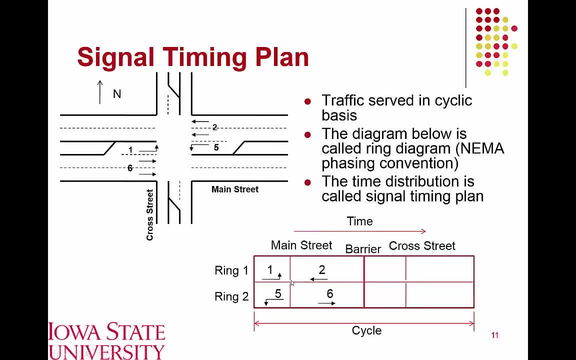 And so when we look at this ring diagram, the left side of the diagram here, when we look at the top and the bottom, the top phase can run simultaneously with the bottom phase, as we see right here. So 1 can run concurrently with 5.. 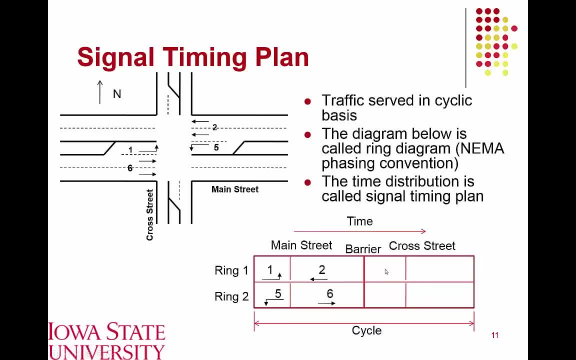 It can also run concurrently with 6.. It's not going to be able to run concurrently with what we see on the other side of this barrier indicated right here, though, because this barrier designates movements 3 and 7, which are left turns on the minor street. 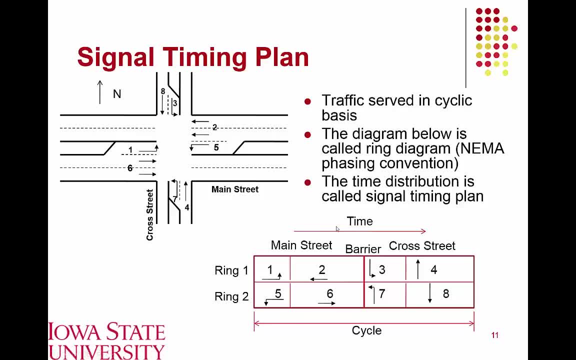 and movements- 4 and 8, which are through movements on the minor street, And so likewise we can shift these barriers to the left and to the right, and 3 can run simultaneously with 7 and 8, 4 can run simultaneously with 7 and 8, so forth and so on. 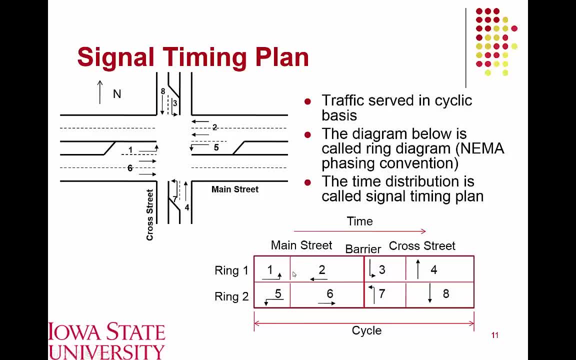 But none of these phases can run concurrently with these phases on the major street. Now, when you're looking at this diagram, you'll notice the main street movements sum to 7, so we have 6 and 1 on one main street and in the other direction we have 5 and 2,. 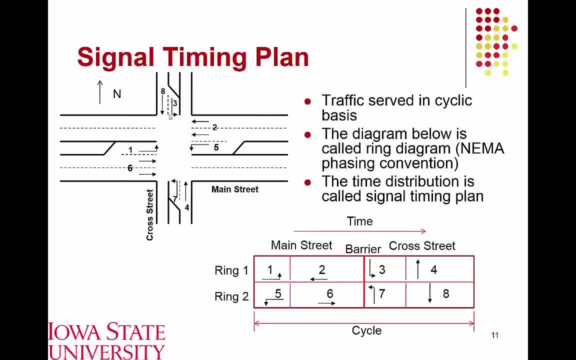 whereas the minor street movements sum to 11.. So we've got 4 and 7 and 3 and 8 in these circumstances, And so what we're trying to do, then, is allocate timing such that we're minimizing delay for these various movements. 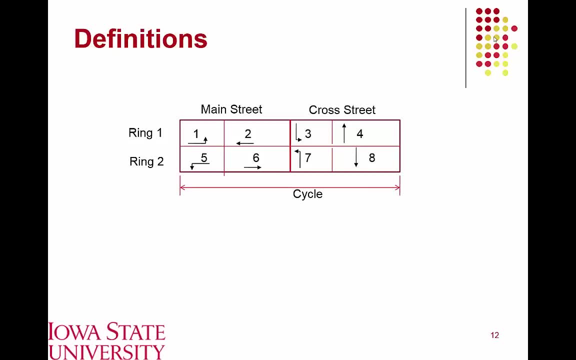 overall at the intersection, And so this is just indicating what we're trying to do here conceptually, And so we refer to each of these boxes here as the split corresponding to a specific movement, And so in this case we have 8 movements. 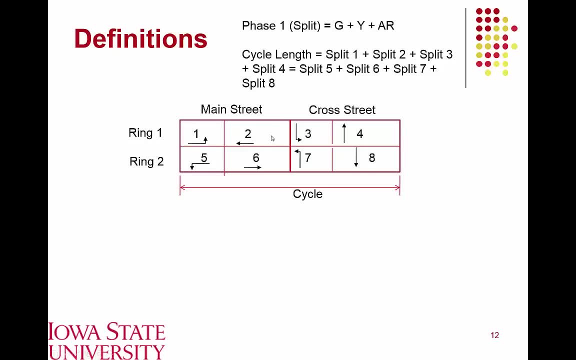 We have 8 splits And so if you sum these- the splits for the 4 movements on the top ring on ring 1, that will be equal to the sum of the 4 movements on ring 2. obviously Just by definition here. 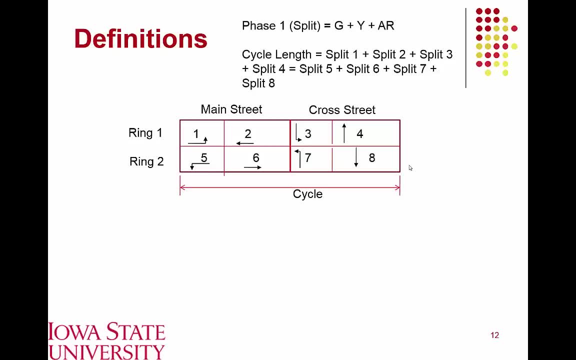 we're going to have consistent signal indications on the major and minor streets respectively, And so what we try to do then is we take each portion of the ring diagram and we're trying to then determine how much time is being allocated to specific movements here. 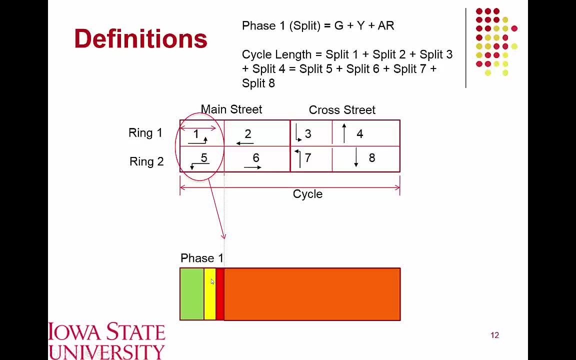 And so we're trying to allocate how much green, yellow and all red time are going to be allocated that are going to be demonstrated for specific movements here, And we do likewise for each of our splits until we arrive at our total cycle length. 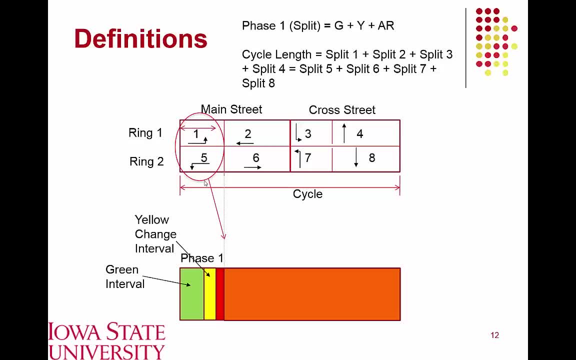 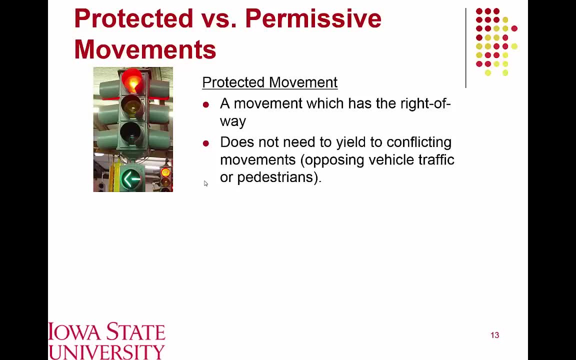 And so from here we indicate the green period, the yellow change interval and also the all red clearance interval. Another concern when we're designing traffic signals is protected versus permissive movements, And we're typically talking about left turning movements at signalized intersections here. 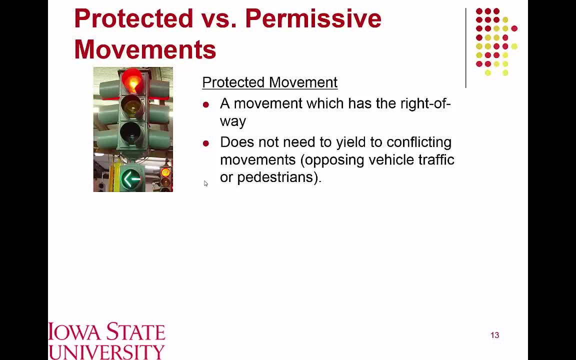 So when we say a left turn is protected, it means that vehicles are able to turn left without having to deal with any potential conflicting traffic coming in the opposite direction, whether that's vehicular traffic or pedestrian traffic, Whereas a permissive movement is an instance. 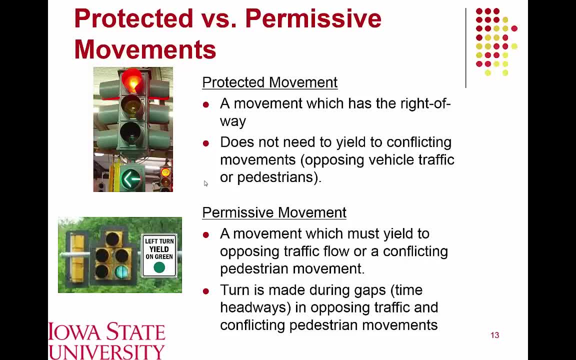 where vehicles have a green indication but they need to wait until there's a gap in traffic coming in the opposite direction. So, for example, as a vehicle is waiting to turn left and they see traffic coming in the opposite direction, that would be an example of a permissive movement. 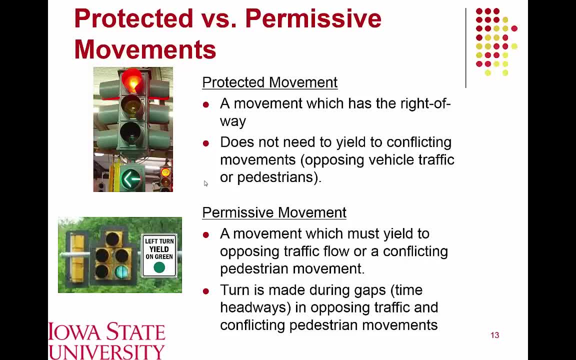 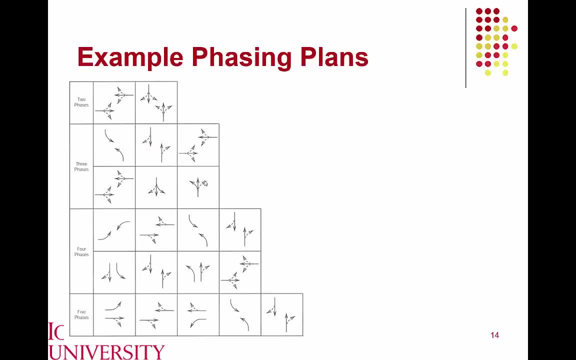 when they can't make that turn until the vehicle is cleared and given them a sufficient turn, And that would be a sufficient gap before the next vehicle arrives. And so these are a few concerns to take into consideration as we develop the ultimate phasing plans. 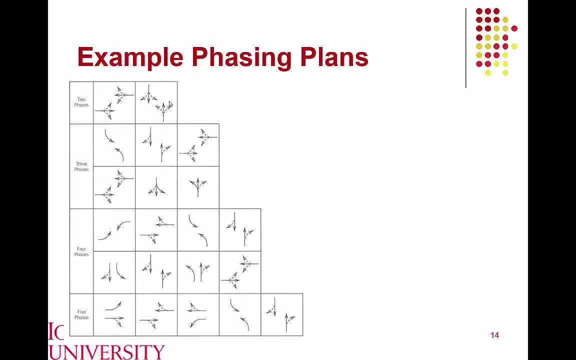 And so what we see right here? in the simplest case, two-phase operation would correspond to a situation where we allow all movements on the major street. so basically, left turns are permitted if gaps are available through movements, and right turn movements can go consistently throughout that entire period. 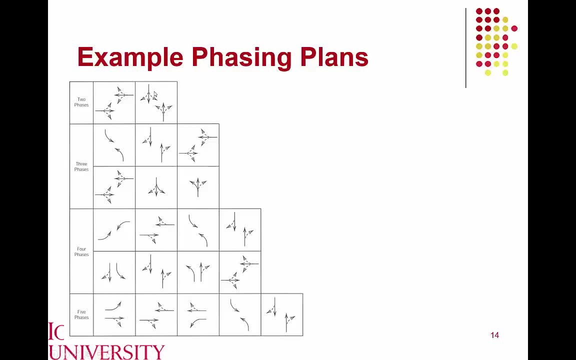 and then we give the signal to the cross street. the cross street has green and the major street. all movements are stopped during that period. We can expand that to three-phase operation. so here we see an example where we have a protected left turn phase. 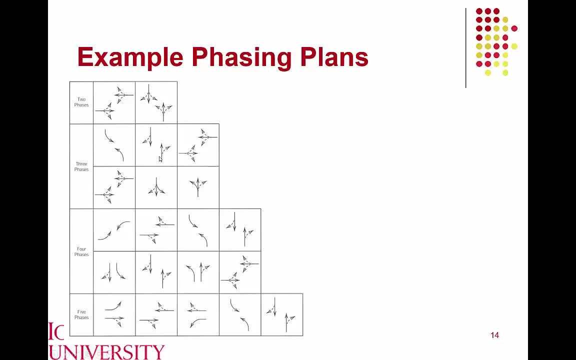 so we start out with only the left turn movements, then we go to the through and right turn movements on the major street, and then the minor street, which is presumably going to be lower volume, allows all movements simultaneously, in which case these left turns would then be permitted and not protected. 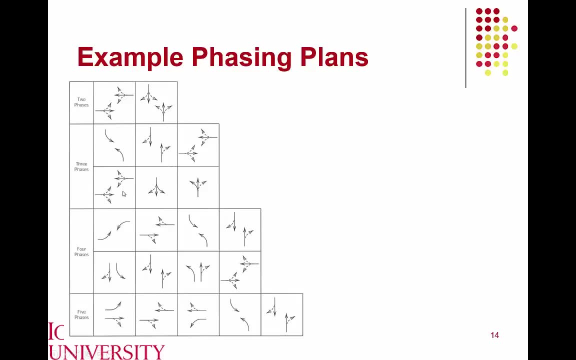 A third example we see here. this is a three-phase diagram where we allow all movements on the major street simultaneously, with permitted left turns, and then we go to what we call split phasing. so then we would allow one direction of the minor street to proceed. 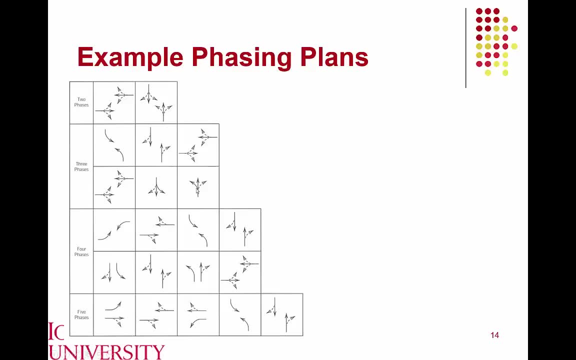 and the other direction of the minor street to proceed and for example, you would see this a lot in Ames where we have relatively high left turning volumes in both directions. so we basically clear out all traffic in one direction of the minor street and then all traffic in the other direction. 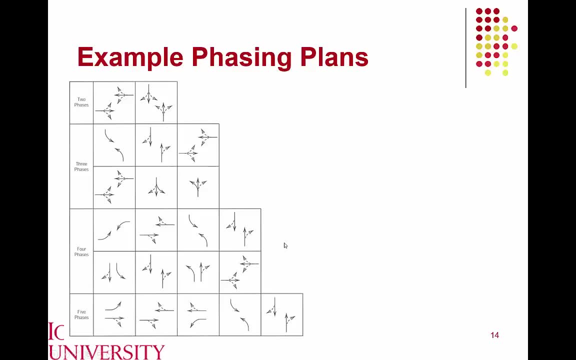 And there are several additional variants here. you see an example where we have leading left turns. left turns are provided, so protected left turns in the first ring of the diagram and then in the second ring of the diagram. we allow different movements that occur during these same periods. 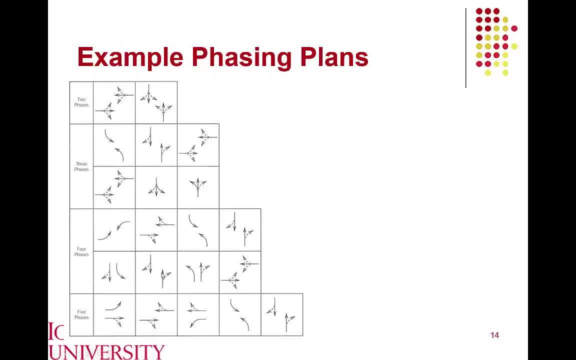 during which we may have permitted left turns on some approaches as well. We also see some examples here for five-phase diagrams as well, and so there are various combinations, obviously, of different phasing plans that we can develop, and this is just again reiterating circumstances. 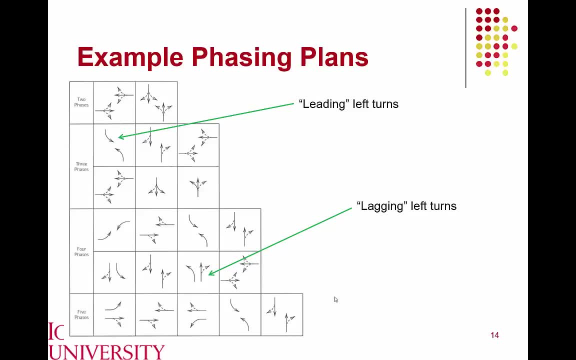 where we have what are referred to as leading left turns and lagging left turns, and so a leading left turn simply means that we're allowing left turns to go first, so they're leading that interval, whereas lagging left turns would be a circumstance as we see right here. 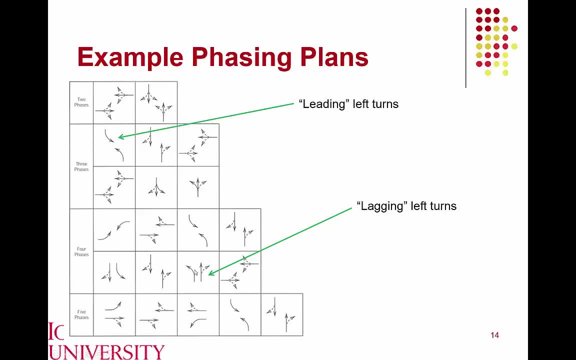 where first of all we're allowing through and right turn movements and then we allow left turns at the very end. so the left turns would be lagging in that phase, And in looking at this we can also look at various combinations. so sometimes your left turns will start out as protected. 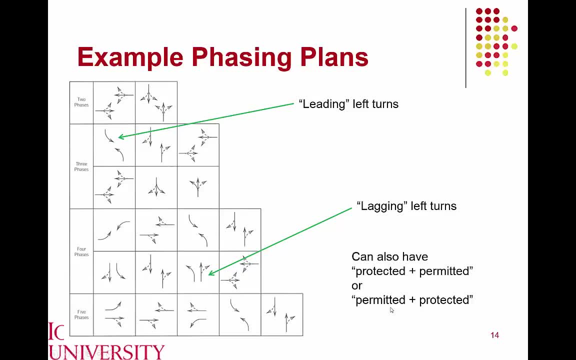 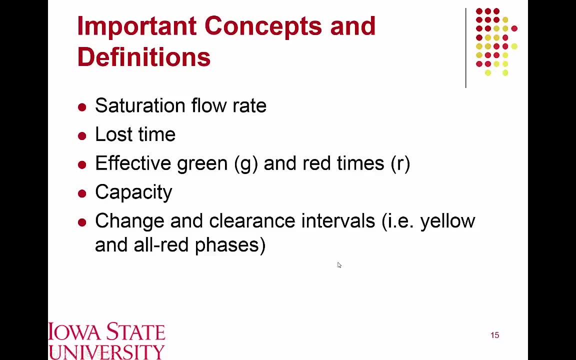 and then they will become permitted. or vice versa: they could start out as permitted and then you would have a protected phase at the end of that phase diagram, as we see here. Now we'll just go through a few of the important concepts and definitions that are introduced in traffic signal design. 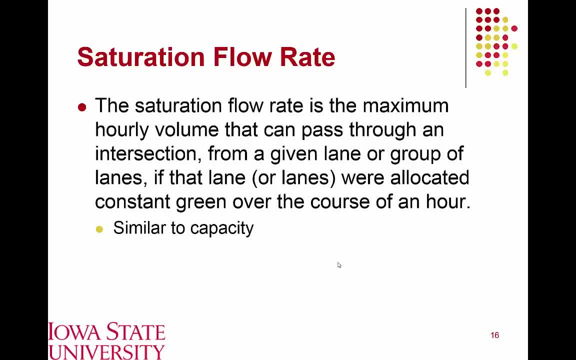 and so going through each of these in order. saturation flow rate is a measure of the maximum hourly volume that we can pass through an intersection within a given lane, So it's very similar to capacity within the context of roadway level of service analysis for various freeway or multilane. 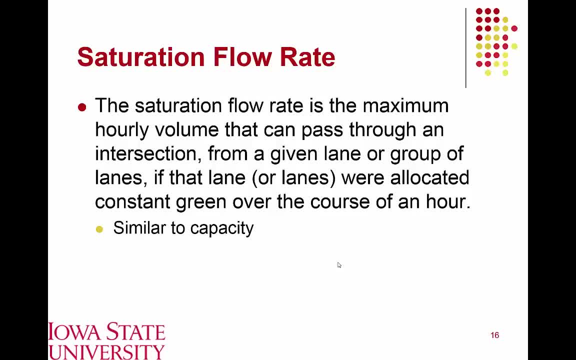 or two-lane highway segments. So we're basically trying to determine the total number of vehicles that can move through an intersection over a given time period, and so the way we do that is based on headway, and so our saturation flow rate is going to be equal to 3600. 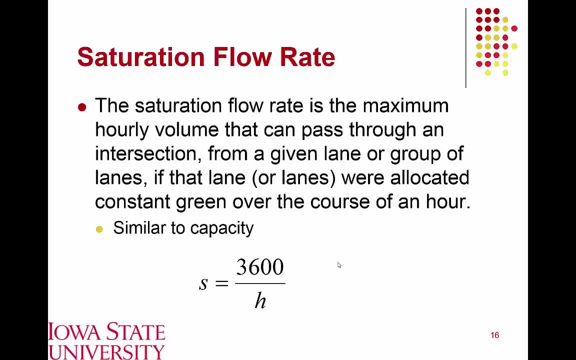 divided by our average headway. So, for example, if you look at empirical research, it'll generally suggest that saturation flow rates will be in the order of 1800, 1800 to 1900 vehicles per hour, So roughly every two seconds. 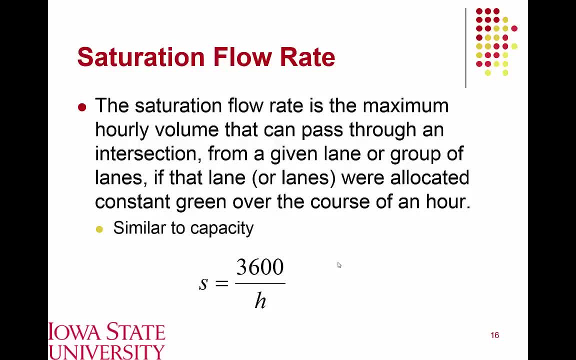 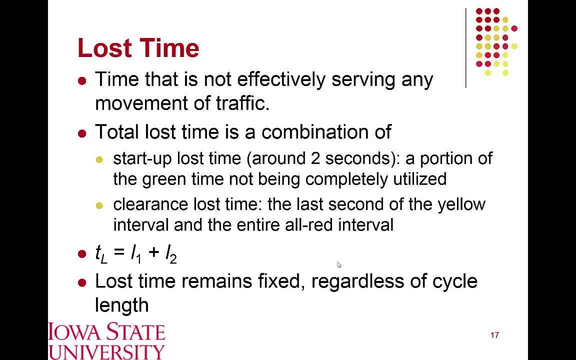 we'd have a vehicle passing through an intersection on a lane-by-lane basis Lost. time is an important consideration when we're looking at traffic signal design. So as a signal goes from green to yellow to red and then back to green, we're not going to see traffic moving consistently. 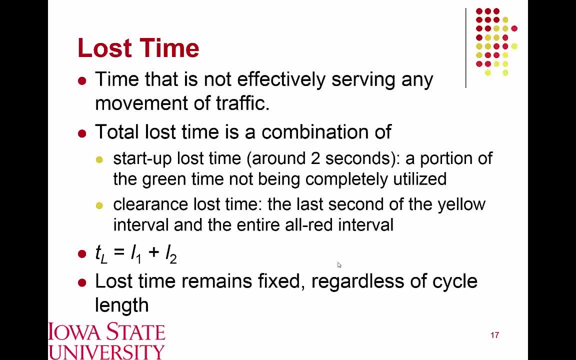 at the saturation flow rate. during those time periods There's going to be slowdown or effectively what we refer to as lost time. So at the start of the signal, when the signal turns to green, it takes a little bit of time for vehicles. 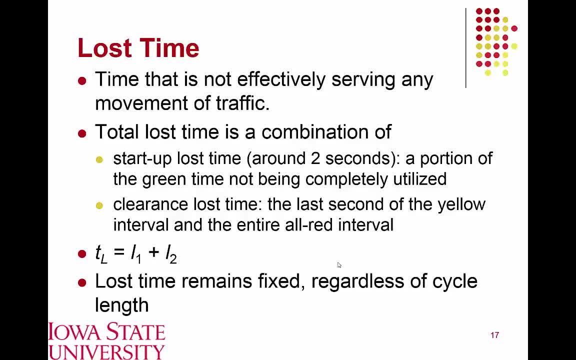 and the traffic stream to get up and moving towards that saturation flow rate, And so we generally assume that takes about two seconds for that traffic stream to start moving- and we refer to that as startup lost time- And then at the end of the interval, 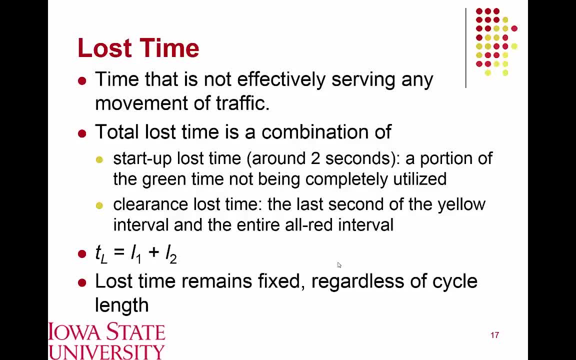 as the traffic signal goes to yellow and then ultimately to red. essentially, that's an unusable time for the movements in that given location, because you're presuming that traffic will begin to stop, and so, consequently, that's a second source of, essentially, time that's lost to the system ultimately. 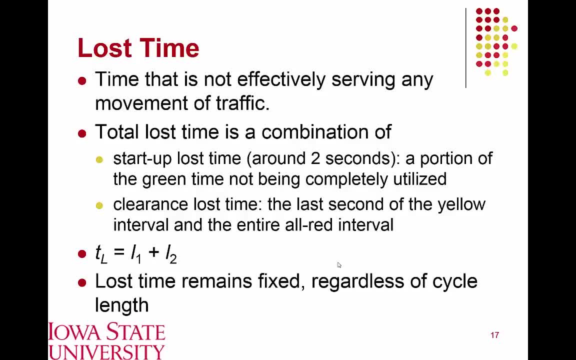 And so when we think about lost time, this is something that's going to remain in the system regardless of what we do with the cycle length. So there's always going to be this lost time that we'll need to account for in signal design. 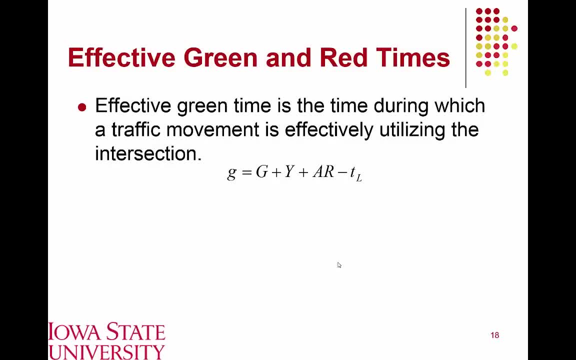 Another important consideration is what we refer to as effective green and effective red times. So the effective green is basically the time during which a traffic movement can actually use that intersection, And so the lowercase g here illustrates effective green, and then the capital letters indicate the green time. 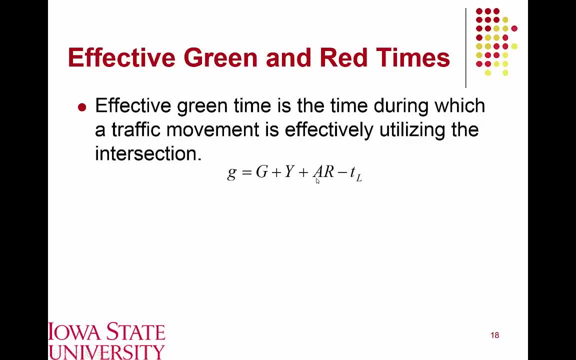 the yellow time and the all red time respectively, And so vehicles have the green movement and can essentially proceed through the intersection, in theory, during the entire green, yellow and then also the all red period. So the all red is referring to the time. 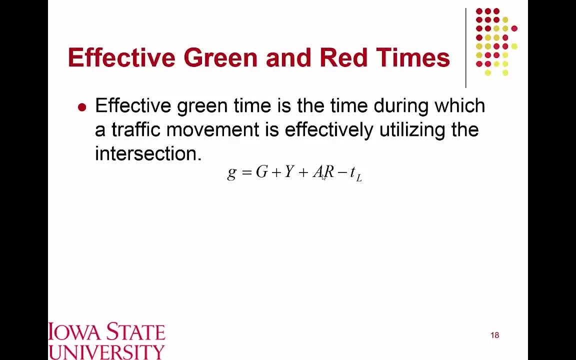 when there's typically one or two seconds provided for red on all the approaches to the intersection. So this isn't the actual time during which we see red only on the effective approach. This is the time during which we see red on all approaches during the signal transition. 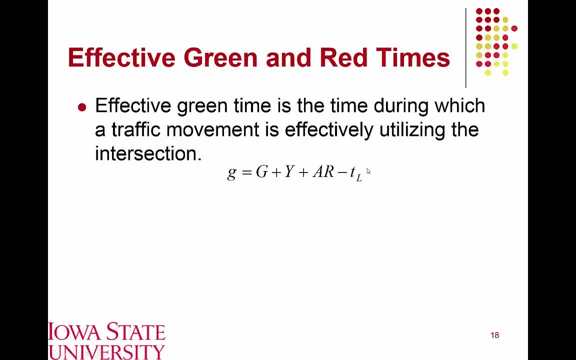 So we take the sum of these three quantities and then we're going to subtract off the lost time, and that gives us our effective green. Now, conversely, effective red is the time during which a traffic movement is not effectively utilized in the intersection. And so, obviously, if we assume that the summation 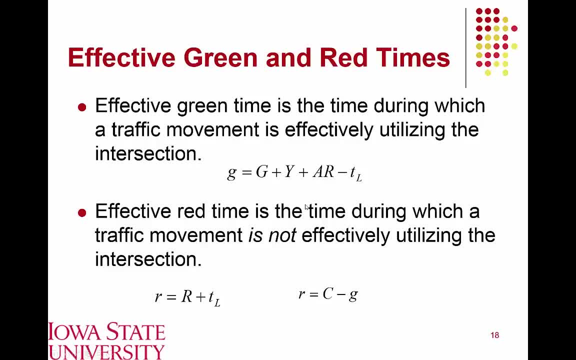 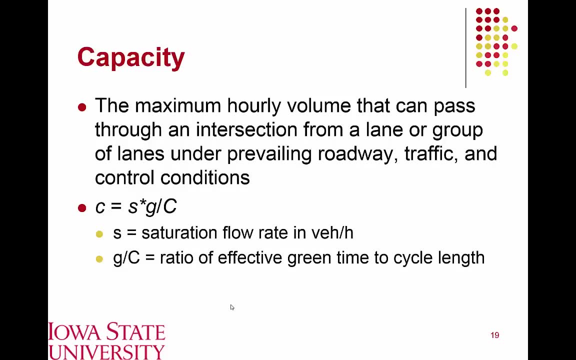 of our green, yellow and red times are equal to our cycle length. our effective red is simply the cycle length minus the effective green, or it's the time period during which a vehicle sees a red phase in addition to that lost time. Now, capacity is similar to what we've seen. 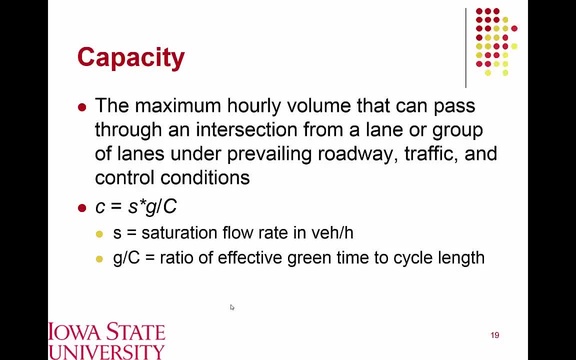 in our prior level of service analyses is essentially telling us the maximum hourly volume that can pass through an intersection during a given time period, And so this is going to relate back to our saturation flow rate. So a few slides ago we had introduced saturation flow rate. 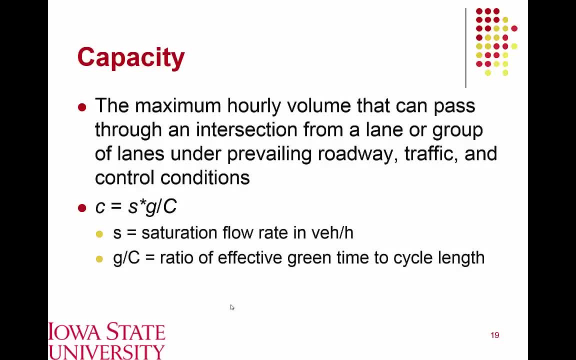 which is essentially the highest volume at which vehicles can move through an intersection during a given time period. Now, if we look at that, or the duration of an entire cycle, so a cycle is basically referring from the time it takes a signal to go from green to yellow to red. 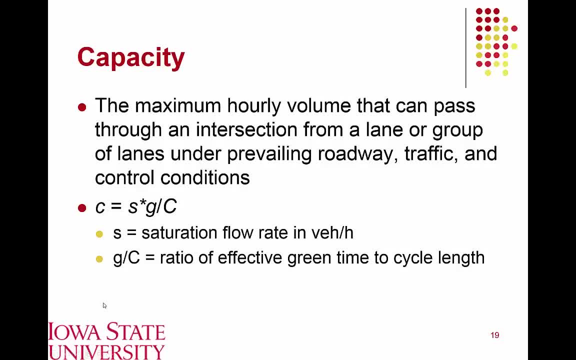 and then back to the start of green again. we just take whatever that saturation flow rate is and then multiply by the proportion of that cycle length that is operating under effective green. So let's say we've got a 60 second cycle If it's green during half that time. 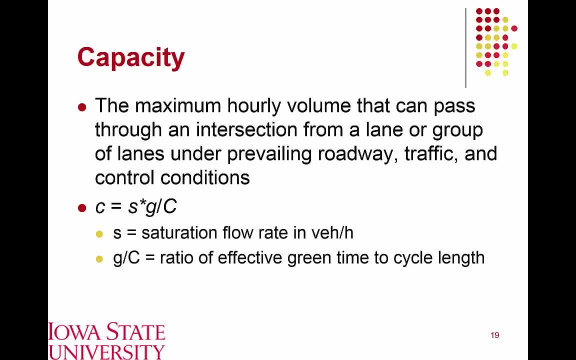 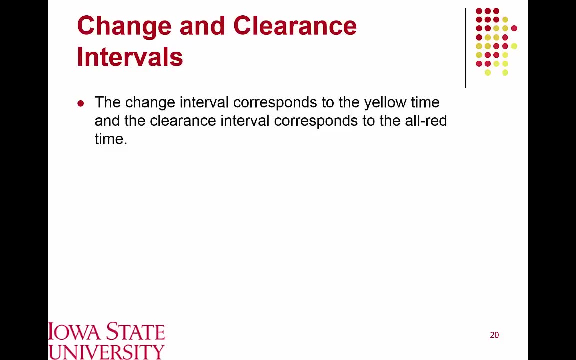 we would be able to serve half of that saturation flow rate over that time period. So our capacity is simply a ratio of the saturation flow rate times. whatever proportion of that time, vehicles are seeing an effective green signal. Related points are the change in clearance intervals. 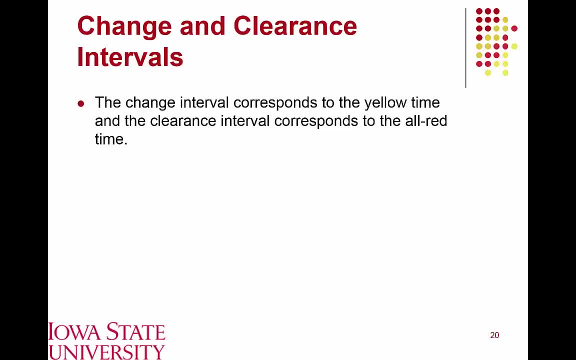 So any time a signal is about to go from green to yellow and then yellow to red, we're going to want to be able to determine what appropriate durations are for yellow time and also all red time, And so typically we're providing yellow time in the range of three to five seconds. 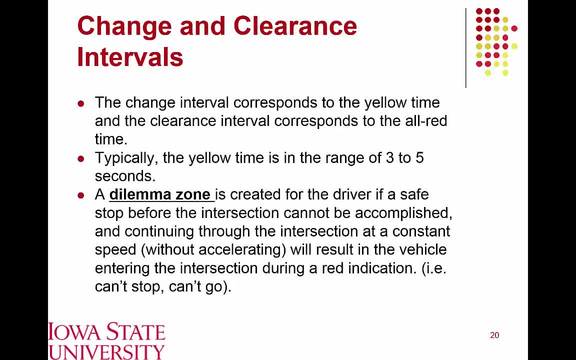 Although one concern we often run into here is drivers can become stuck in what we refer to as a dilemma zone. So basically, the light goes from green to yellow. They're too far from the intersection so that they can proceed through safely, but they're also too close, such that they can stop safely. 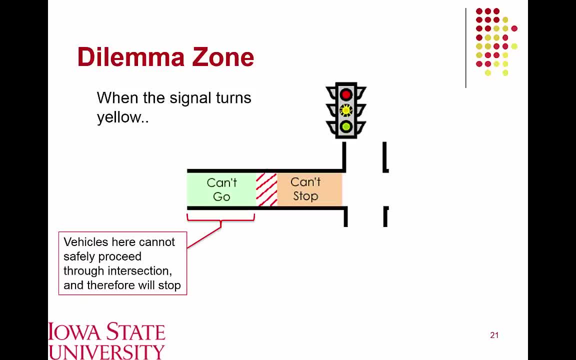 And so, if we look at this schematically in this diagram right here, if you get to the intersection far enough in advance, when the signal goes from green to yellow, drivers can obviously stop safely before getting to the intersection. Likewise, if they're too close to the intersection. 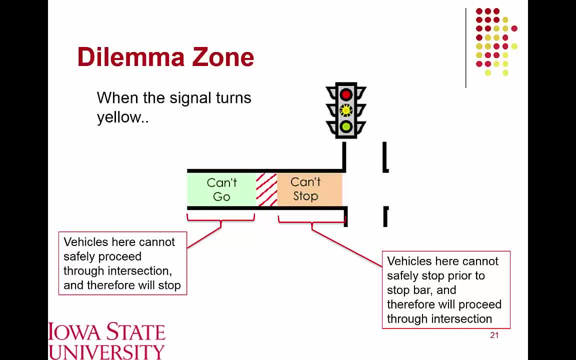 when that light goes to yellow and then to red, they're not able to stop, but they're able to proceed through safely. The dilemma zone is this time in between, when we're kind of in the fringe, and then, based on the underlying physics, 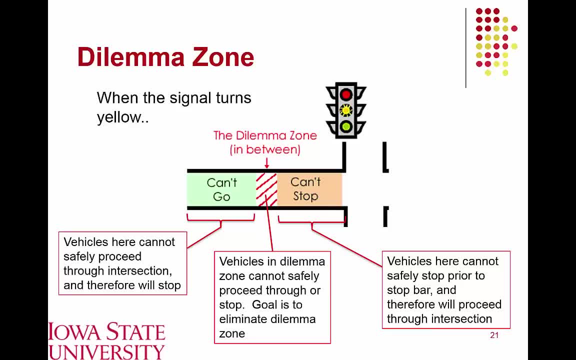 we're too close to safely stop, and yet we're too far, such that we can safely clear the intersection before it goes to red, And so what we try to do is we try to minimize this time for vehicles in our system. So, in order to determine appropriate lengths, 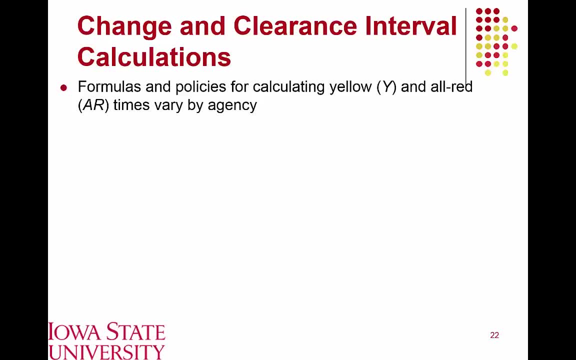 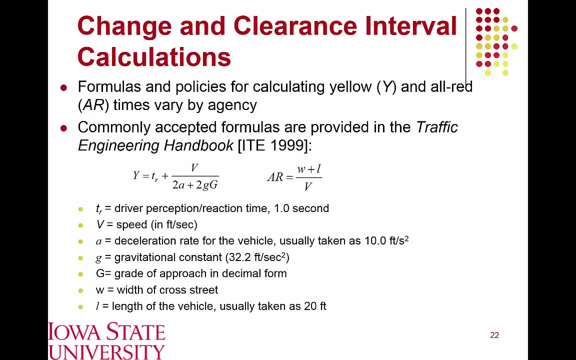 for the yellow and all red times. this is often going to vary by agency, but the Institute for Transportation Engineers offers some recommendations here, So the yellow time is simply going to be equal to reaction time. since this is an anticipated event, Drivers are familiar that that signal may transition to yellow. 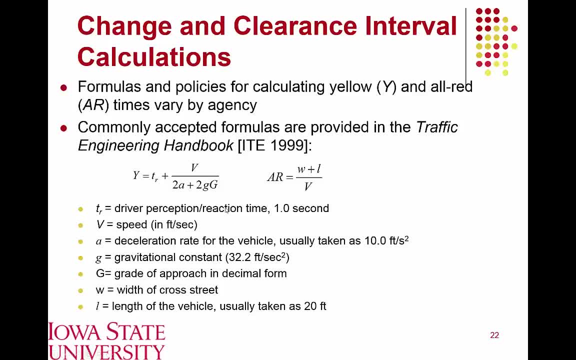 We're going to assume one second reaction time here, and then we're simply looking at the velocity or speed of that vehicle divided by 2 times the deceleration rate, which we're generally assuming to be 10 feet per second, squared, plus 2 times g, which is our gravitational constant. 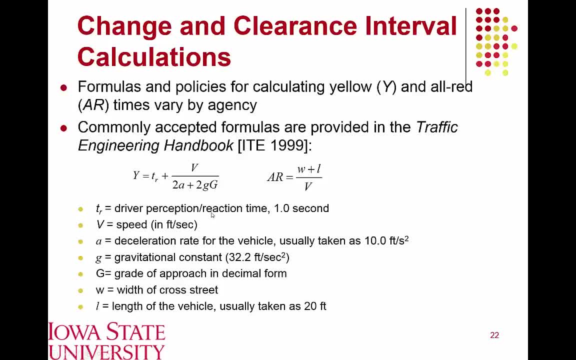 and a second g here, which denotes our grade, And so what this is essentially telling us is that we need to provide more yellow time to accommodate higher speed locations and also determining what our grade is. So if we're on a downgrade and it takes a longer time, 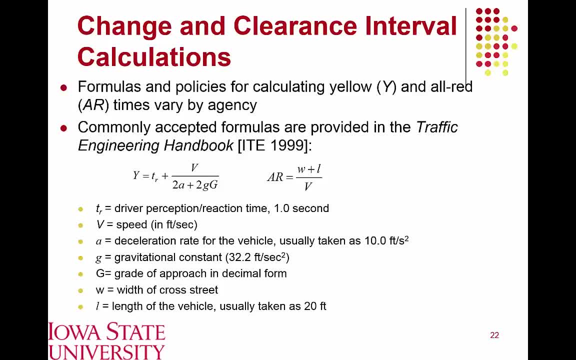 for vehicles to stop, we would obviously need to provide a different yellow time than if we were on an upgrade and that vehicle would not need as much time to stop. ultimately, On the right side here, this is our calculation for the length of our all red phase. 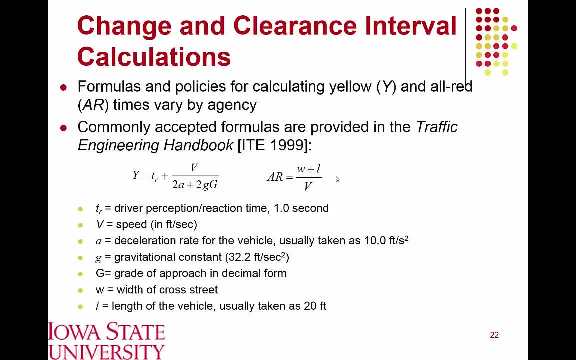 And so here we're concerned with the width of the cross street. so how far does that vehicle need to go to clear the intersection? And then, secondly, what's the actual length of that vehicle? So if we take those respective lengths and divide by whatever the design, 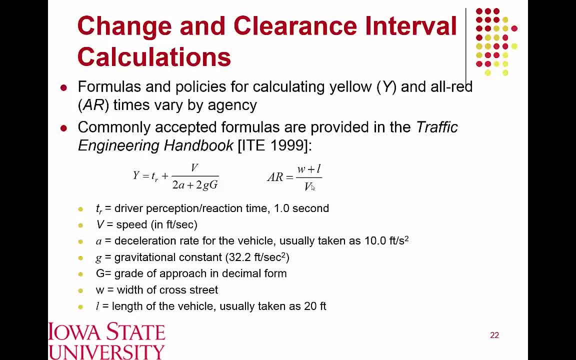 or operating speed of that facility is that's going to give us an all red time, which is basically a safety buffer, because you're assuming not all vehicles are going to clear through prior to the start of red, so this is a buffer time before that cross street goes to green. 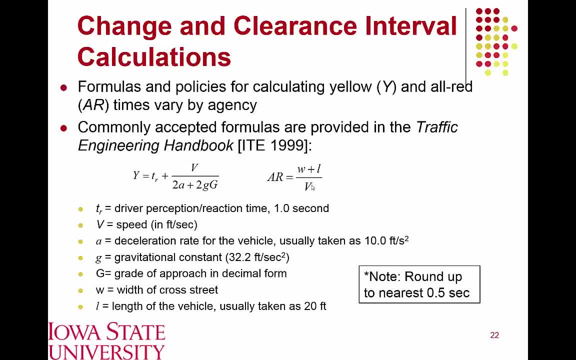 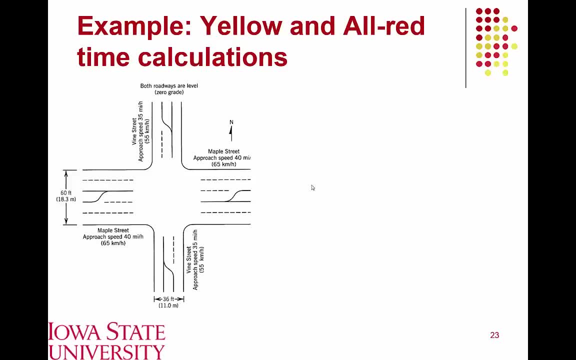 Typically, as practice, we will round this up to the nearest 0.5 seconds when calculating the yellow and all red times, And so, as just a quick example here we see yellow and all red time sample calculations. So we have a major street posted. 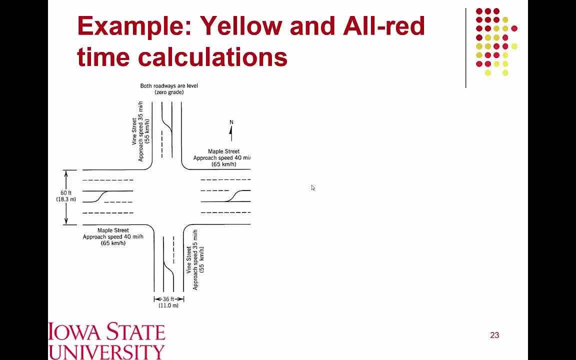 at 40 miles per hour, a minor street posted at 35 miles per hour. We're assuming level grades and the minor street is 36 feet in width. the major street is 60 feet in width, And so to cross on Vine Street we have one second. 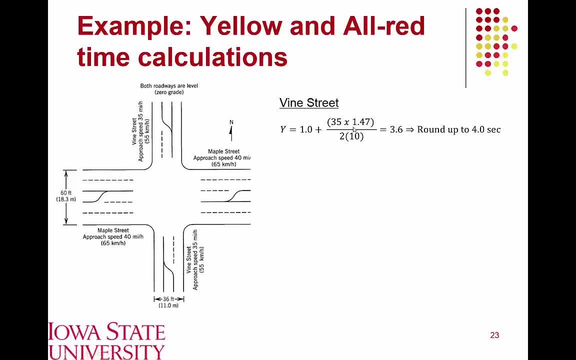 plus the 35 miles per hour, which we're converting from miles per hour to feet per second here, with the 1.47 divided by 2 times our acceleration rate, gives us 3.6 seconds, and so we're going to round that up to four. 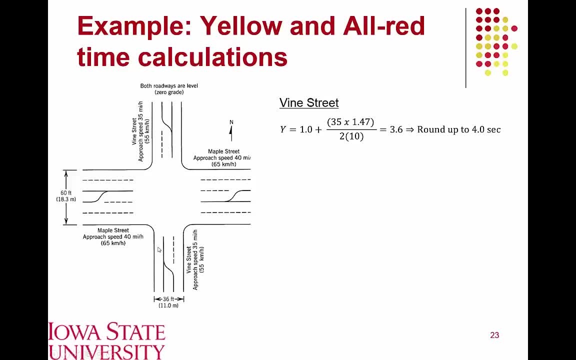 Okay, so the vehicles are waiting to cross through this intersection, and so we're providing four seconds of yellow in that circumstance. In the case of the all red phase, we see it's needing to cross a street that's 60 feet wide. 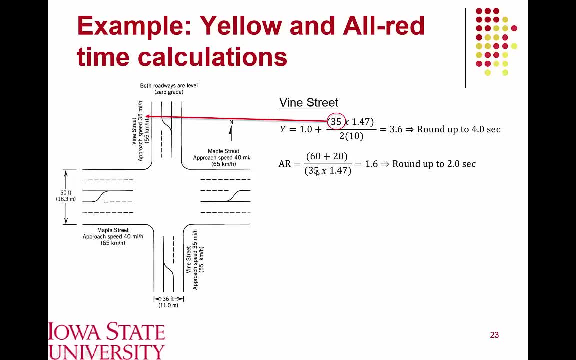 We're assuming a 20-foot vehicle width and so, assuming that same 35 miles per hour, which we're converting to feet per second, we get 1.6, which is then rounded up to two seconds. Looking at the main street in this section. 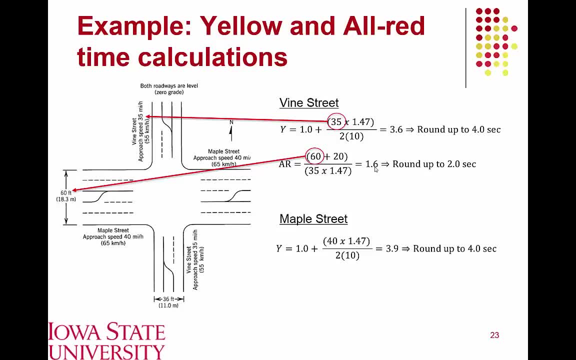 we see that in this circumstance, using similar calculations, we have a higher speed. in this case, we're still rounding up to the same four seconds for yellow time and the all red time. in this circumstance, since the speed is higher, we don't need quite as much time.